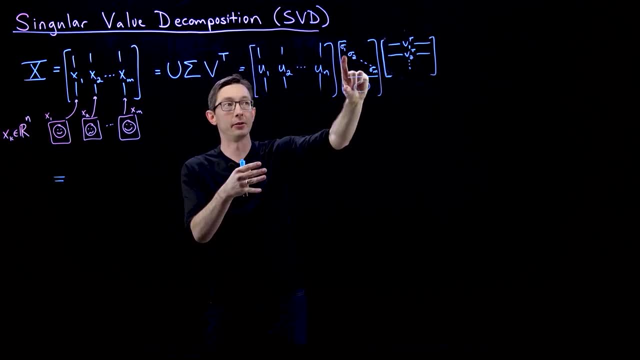 It only gets multiplied by sigma one because every other term in this column is zero. So if I take that and multiply it, it multiplies this by sigma one, all of the others by zero. Same with the second column. It gets zero, U1 plus sigma two, U2 plus zeros of. 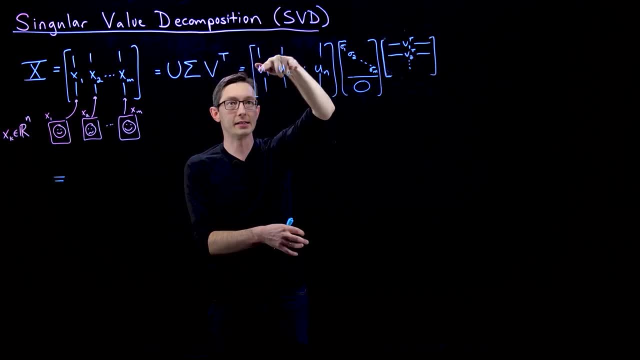 everything else And so on and so forth. So this essentially is: if I multiply this, I get sigma one U1,, sigma two U2, and so on and so forth. And then, similarly, if I take that matrix and I multiply it, 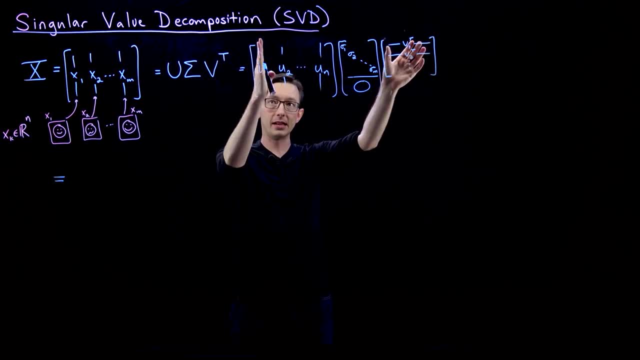 by this V transpose matrix, the first column, sigma one, U1, only multiplies the V1 transpose column, The second column only multiplies the V2 transpose column, and so forth, And so what I end up getting is an expansion that looks like: 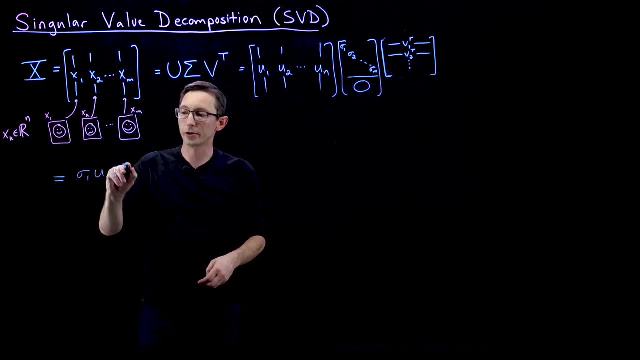 sigma one, U1, V1 transpose. that's the first column, is this times, this times this, plus sigma two, U2, V2 transpose. And I encourage you to actually multiply this out this times this and then that times this, and you'll see that you get. 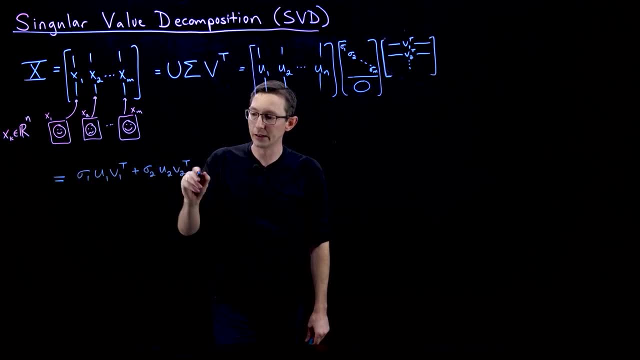 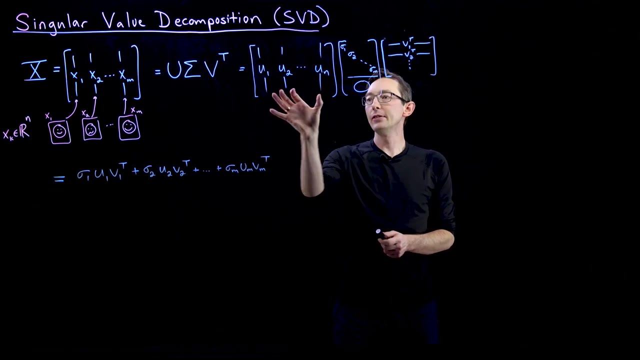 this expansion: Sigma one- U1- V1, plus sigma two- U2- V2, plus dot dot dot. Eventually you'll get sigma M- U2- V2.. Sigma one- U1- V1- transpose- And here's where it gets interesting- Even though this U matrix has N columns, so it's a massive N. 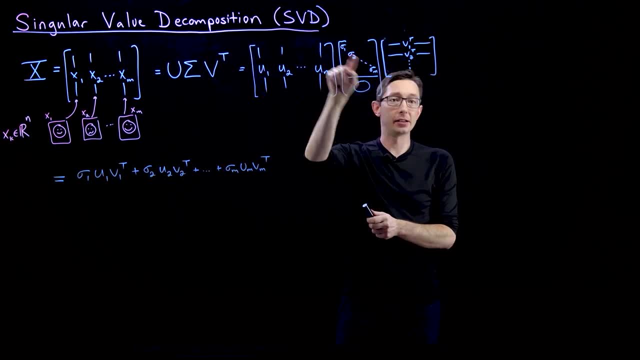 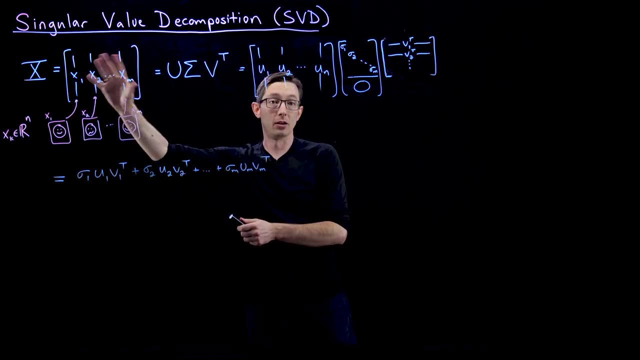 by N matrix. there are only M non-zero singular values, because this thing can only have at most rank M. There's only M linearly independent rows and columns of this data matrix X. And so, even though I could keep writing this out, plus sigma M, 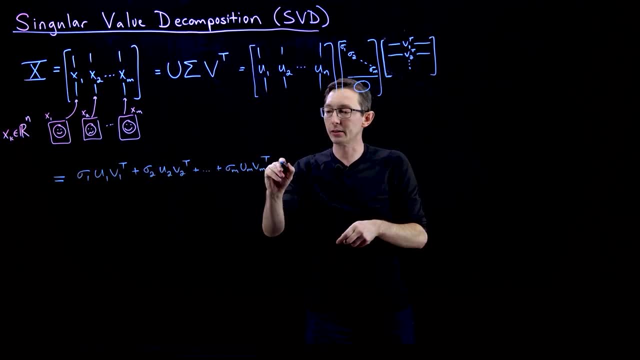 plus one, U M plus one and so on and so forth. all of those singular values are zero. So everything after the first M columns of U and V get multiplied by a zero. So I can throw all of those away, And essentially what that means is that I can select just the 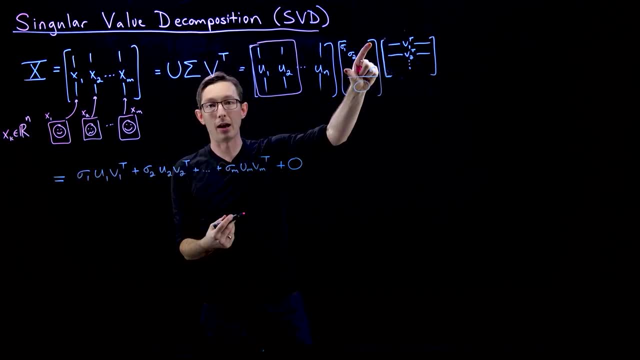 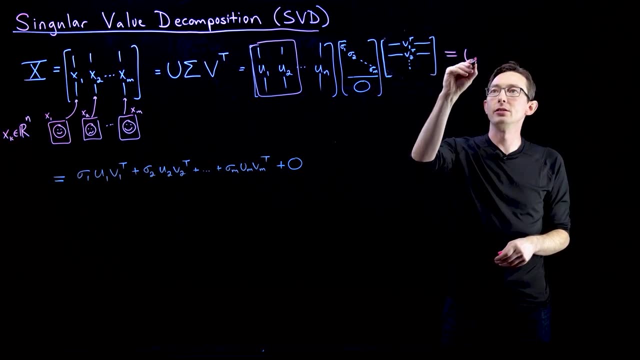 first M columns of U, the first M by M, block in sigma and the M by M, matrix V, And that equals: we're going to call this U2, U hat, sigma hat, and I actually didn't do anything to V. 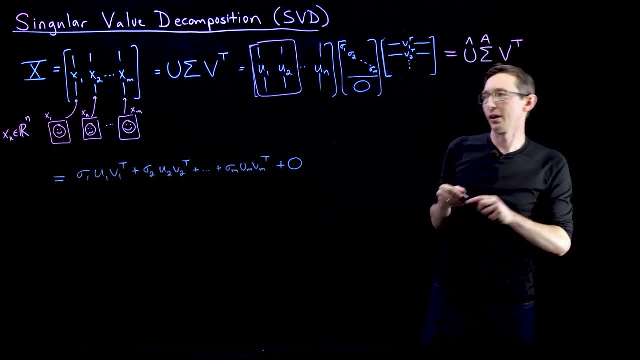 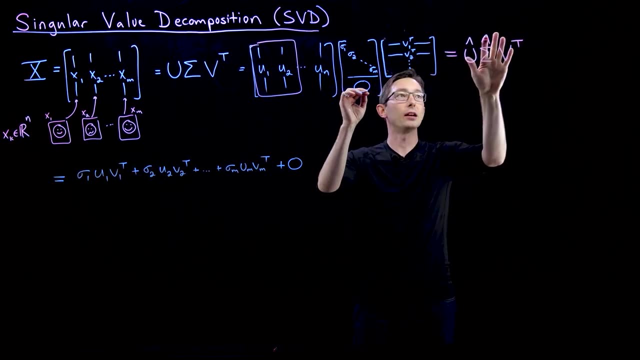 It didn't change at all, V transpose. So U hat and sigma hat are just the first M columns of U and the first M by M block of sigma And V is the original V matrix, And this is exact. X is equal to U sigma V transpose and it's also exactly equal to U hat. 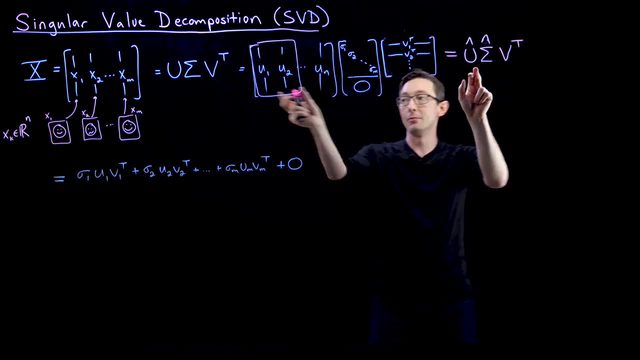 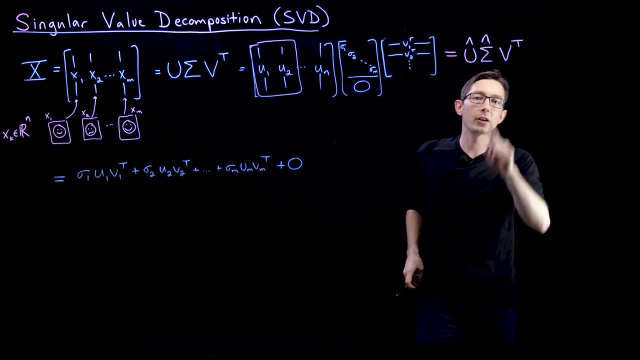 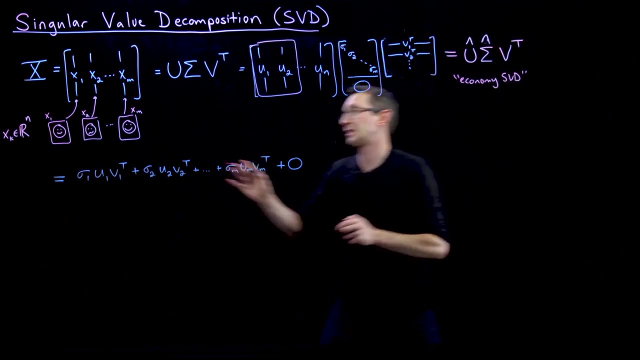 sigma hat V transpose, where these are just the first M columns of U and the first M by M matrix of non-zero singular values. This is often called the economy SVD, And it's actually what you want to do in almost all cases. 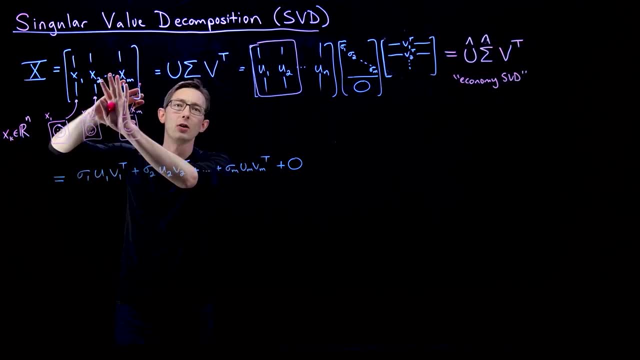 especially where you have tall skinny matrices. I've been assuming the whole time in these lectures. what I've been assuming is that N is much, much larger than M, meaning I have a lot more measurements, maybe a megapixel, million measurements in. 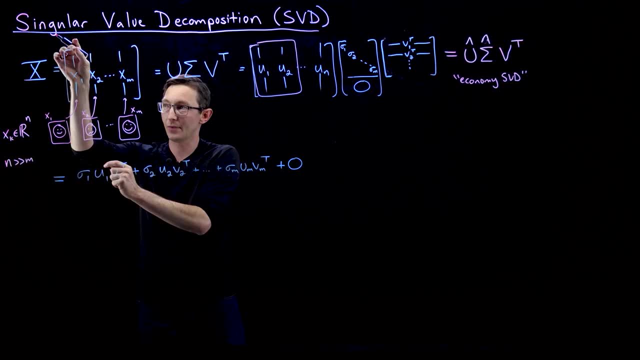 each column. I have many more entries in each column than I have number of columns. So maybe I have a million pixels per column, but I've only got a few hundred or a thousand people, So this would be a million, this would be a thousand. 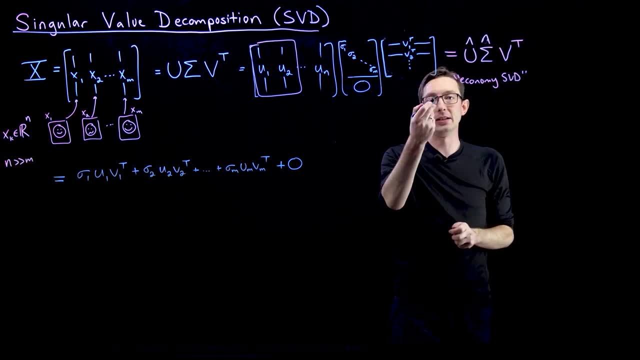 That's what I've been assuming, And in that case you want to run the economy SVD. So in MATLAB again, this is U S, V equals SVD. Okay, Cool SVD of X, but now you give it the econ option. 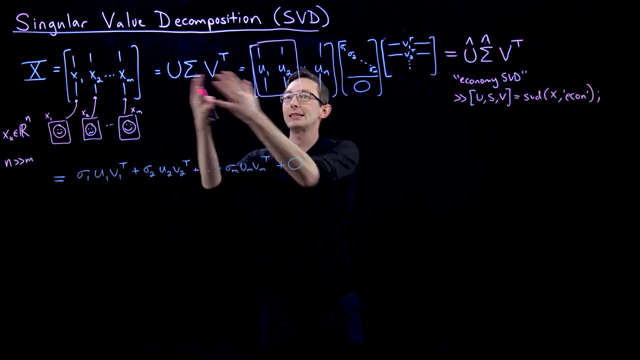 Okay, And what that does is, instead of returning this massive N by N U matrix with all of the complete basis, all N columns of U, what it does is it only returns the first M columns of U that are corresponding to this part, that have non-zero singular values. 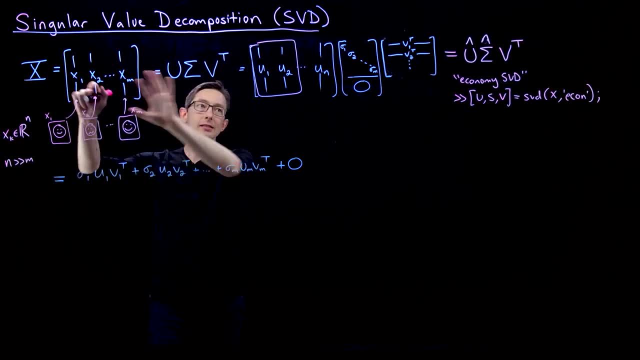 Okay, Good. So you want to expand your X In terms of these rank one matrices. So I'm saying: this is a rank one matrix, this is a rank one matrix, and so on and so forth. So the way you see that is as follows: 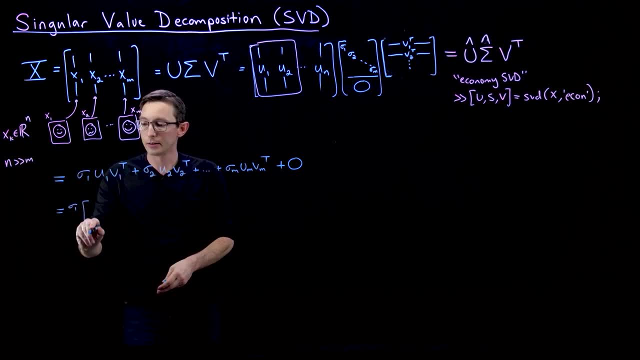 So U1 is a column vector. This is sigma one times my column vector U1 times my row vector V1. transpose: This is U1, V1. transpose plus sigma two: again: column vector U2, row vector V2.. transpose plus dot, dot, dot plus all the way up to Sigma M. column vector UM row. 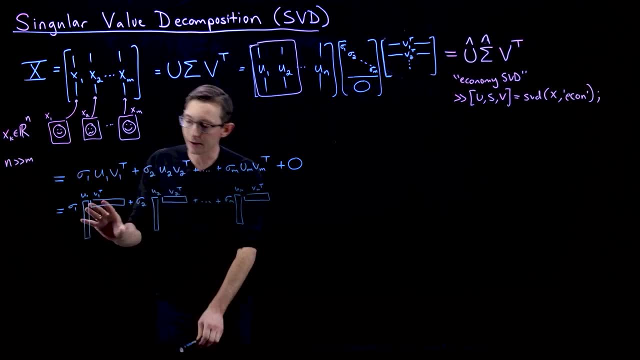 vector VM transpose, and so you can. you're probably used to computing vector vector products like inner products, where you have a vector on its side times, a tall vector, something like that. this is called an outer product, but it's totally fine, what you do. this is a matrix. what you do is you take the first. 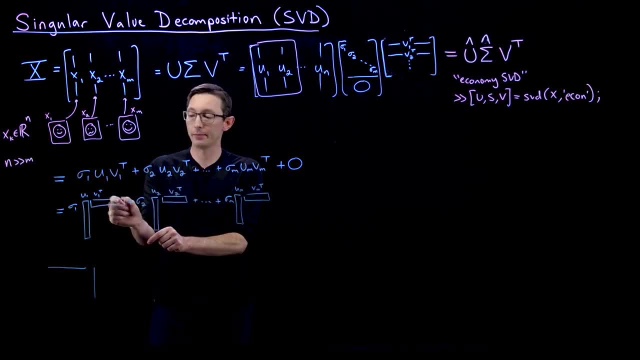 element of you one and you multiply the whole vector view on by that. that's the first row. the next row is the second element of u1 times that whole row v1 transpose, and so on and so forth. you just go element by element and you multiply this row by that element, this row by that element, this row by that. 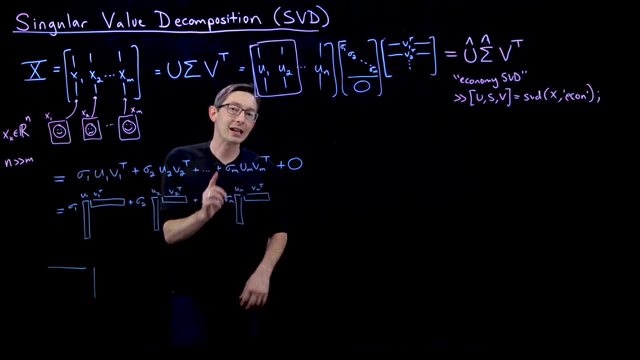 element, and so on and so forth, until you get a matrix. now I say it's rank one because that matrix, by construction, has exactly one linearly independent column and linearly independent row. every row and every column of this matrix is dependent on this row and this column. so this is a rank one matrix, this is a rank one matrix, and so on and so forth. okay, 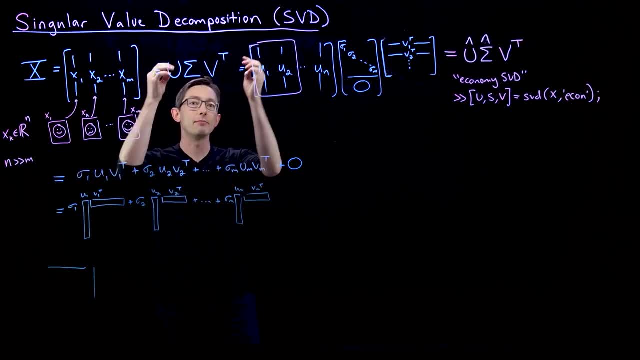 so that's another interpretation of the svd. is that what you're doing is you're decomposing x into these orthogonal bases, u and v, where essentially you can write this as a sum of these, these rank one matrices that increasingly improve the approximation of x. so if i only got one vector, 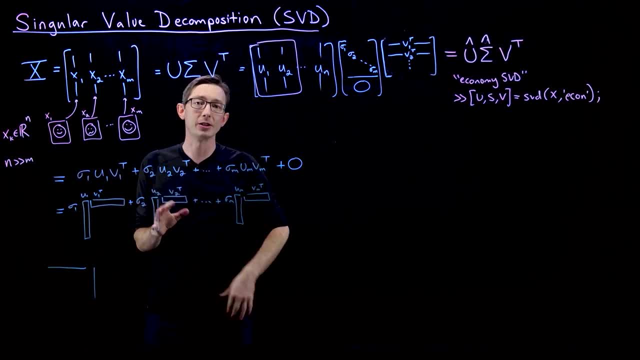 u and one vector v. the best rank one approximation i can possibly make to my matrix x is this one here: sigma u1, v1, transpose. if i get another column of u and column of v, i get to add this: sigma u2, v2, transpose. this is the next best. uh, this is the best rank two matrix that approximates. 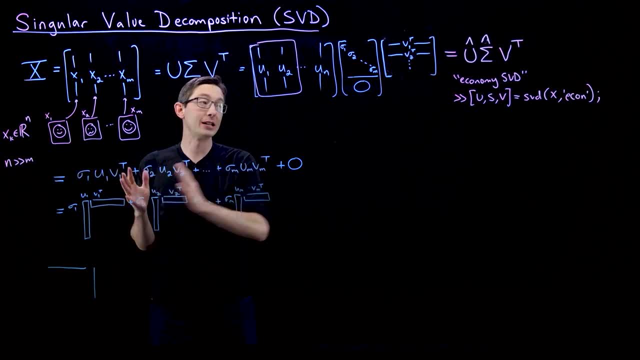 x, and the best rank, three and four and five are obtained by keeping the first three or four or five columns of u and v. okay, so that's that's what the singular value decomposition means. and again, oftentimes what we'll do is we'll truncate, we'll truncate. 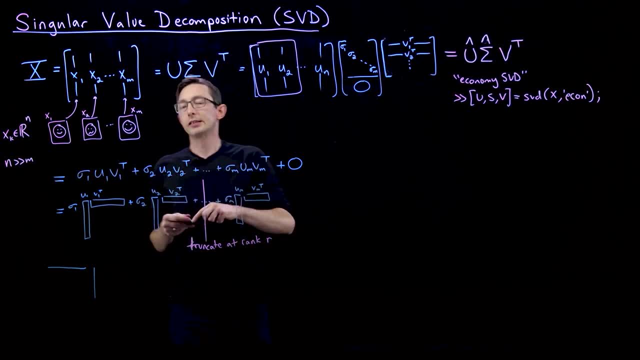 at rank r okay. so oftentimes if i have a lot of really small singular values, like, let's say, sigma r plus one and r plus two, all the way down to sigma m, are really, really small, negligibly small, and most of the information of x is captured in the first r: singular values and singular vectors. 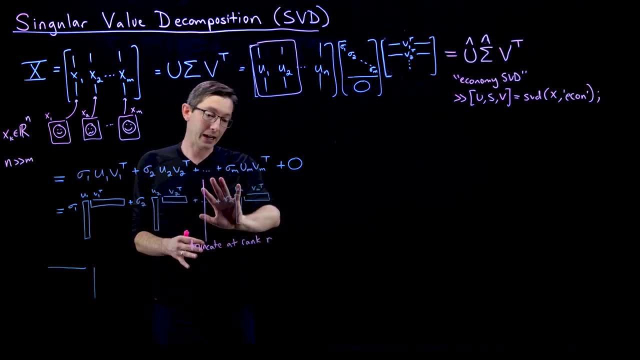 then what i can do is i can chop this summation off and i can throw away all of the low energy singular values and only keep the first r columns of u and r columns of v and r by r sub matrix. so let's now say that this is a little r by uh, the first r columns. 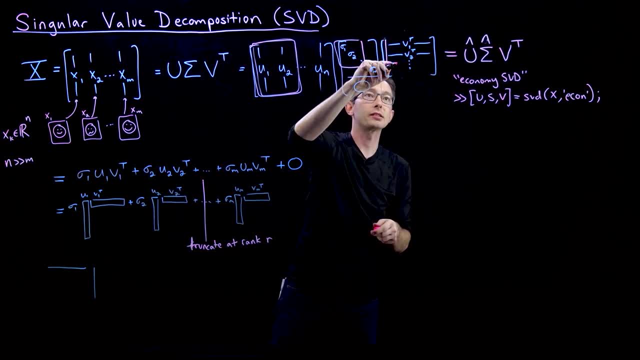 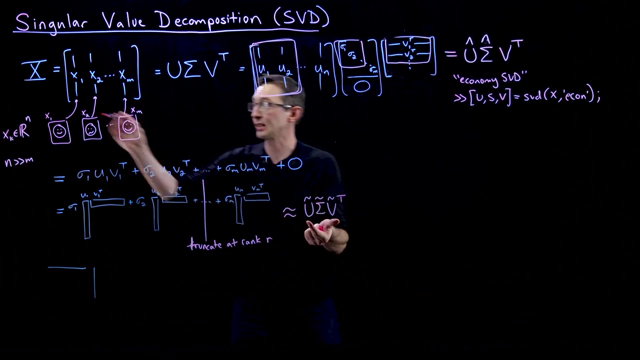 i keep a little r by r and i keep the first r rows of v transpose that we're going to define as u tilde, sigma, tilde, v, tilde, transpose. okay, and here i've said that x is only approximately equal to this, because this is a rank r approximation, this is the best approximation of x. 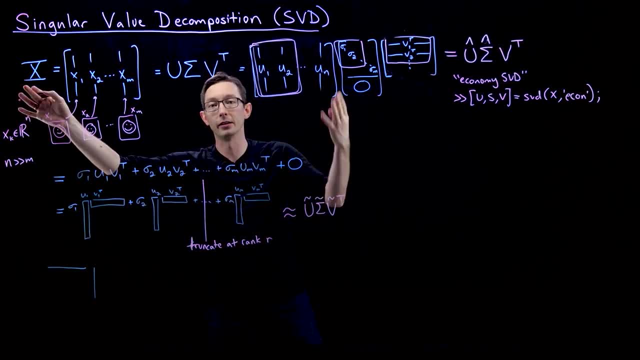 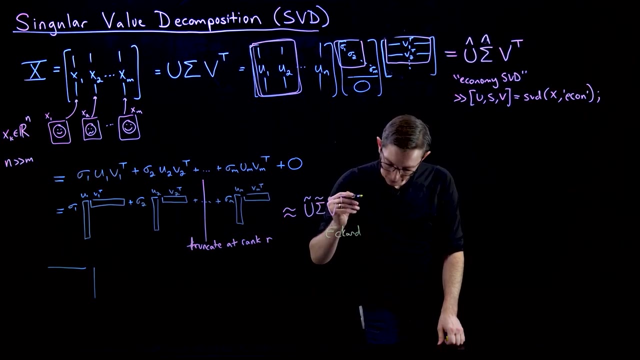 with of rank r in terms of r, column r linearly dependent on r, independent rows and columns. okay, and in fact this has been formalized in a theorem by eckert and young. so this goes way back, the eckert young theorem, eckert young theorem. and this is in 1936. so all of this theory goes way, way back over 100 years for. 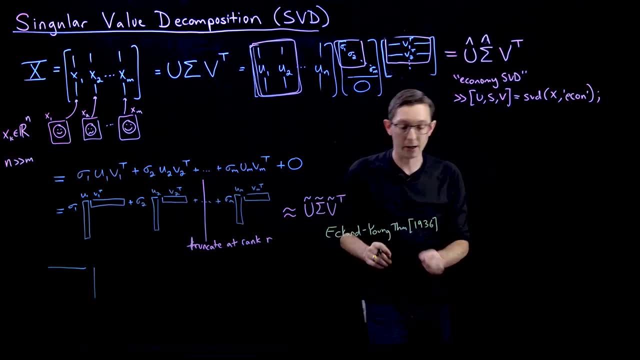 the, the singular value decomposition, almost 100 years for the eckert young theorem, and what it states is that the square root of n is equal to the, including the. the forgot expression for e, a, the, is that the absolute best approximation to the matrix X that has rank R? 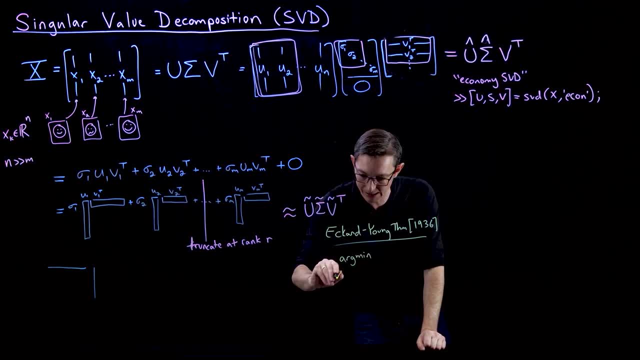 so the arg min the best X tilde, such that rank X tilde equals R. the best X tilde that minimizes X minus X tilde in the Frobenius norm is given by: and what arg min means is that whatever argument minimizes this. 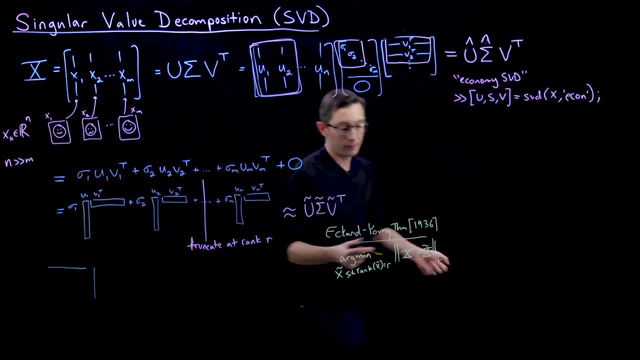 whenever X tilde does have the smallest error and has rank R is the output and that is exactly equal to U tilde, sigma tilde, V tilde transpose. So the Eckert-Young theorem essentially guarantees that the best possible matrix approximation to X of rank R 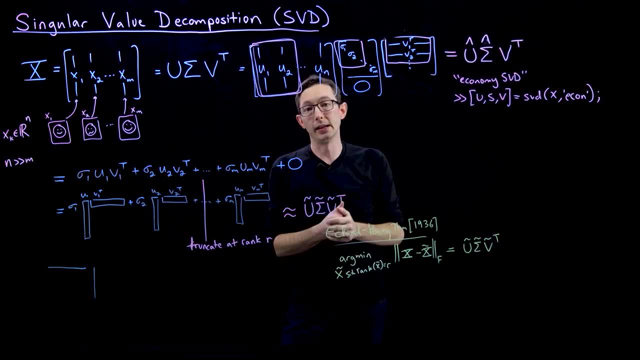 is given by the first R truncated singular value decomposition. You take the first R columns of U, the first R columns of V, and then you take the first R columns of Y, and then you take the first R columns of Y, and then the first little R by R. subblock of sigma. 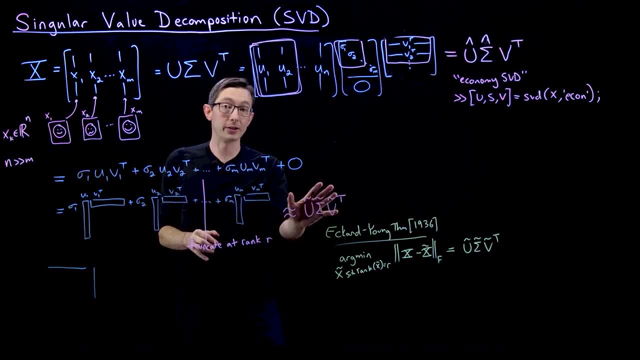 and you can approximate this matrix X very accurately and efficiently in terms of that truncated SVD. Okay, very good, And we call this U, tilde, sigma, tilde, V, tilde in the book. Now, one last thing I want to point out is that, before remember, this U and this V are actually unitary. 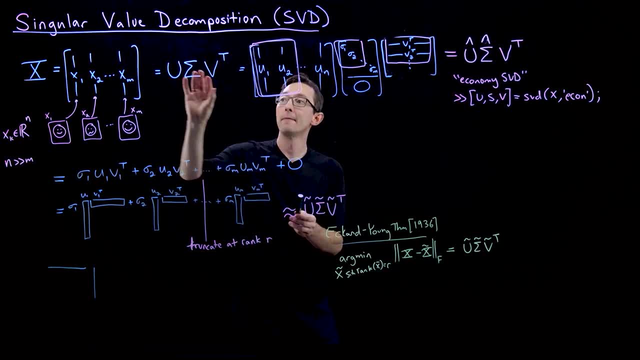 This is an N by N matrix, This is an M by M matrix. And if I multiply U, U transpose or U transpose U, I get the identity matrix. But here, if I truncate at rank R, if I throw away some of the columns of U or V, 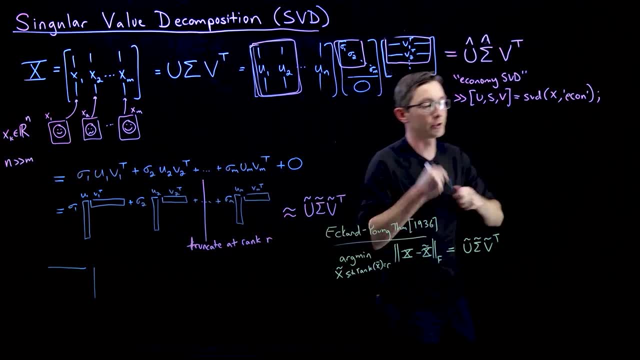 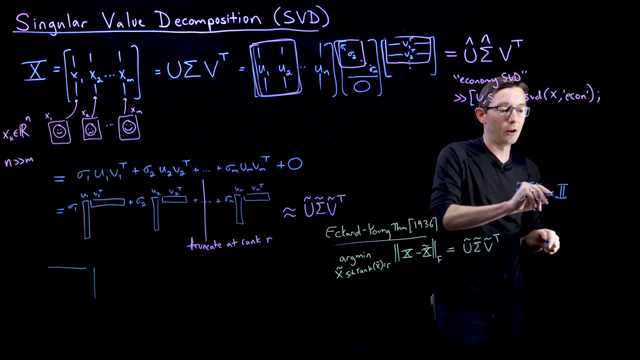 now these are no longer square matrices, And so this is not exactly true anymore. It's still true that U tilde transpose U tilde is the R by R identity matrix, But it is not true that U tilde, U tilde transpose. 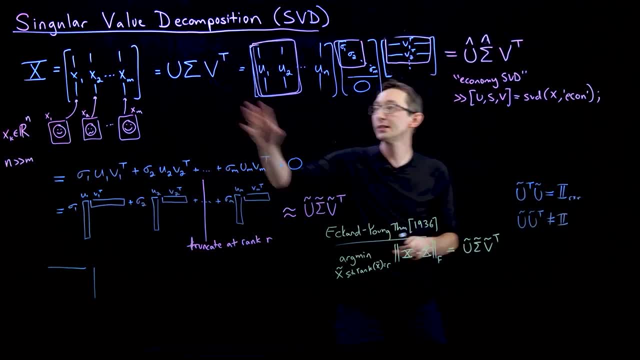 this is not an identity matrix. Okay, so it was before truncation, but after truncating: U transpose- U is an identity matrix, but U U transpose is not the identity matrix, And this is really, really important. Lots of us are guilty of forgetting this basic, basic fact. 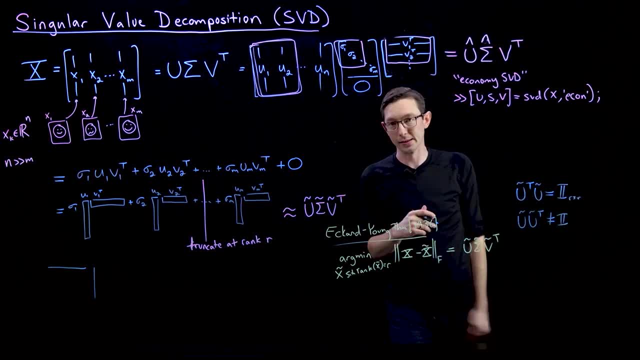 and having wrong proofs because we just forgot that this is true. I'm guilty of this as well. U transpose- these columns are still orthogonal. So if I take U tilde transpose looks like this If you knock these columns over on their side: 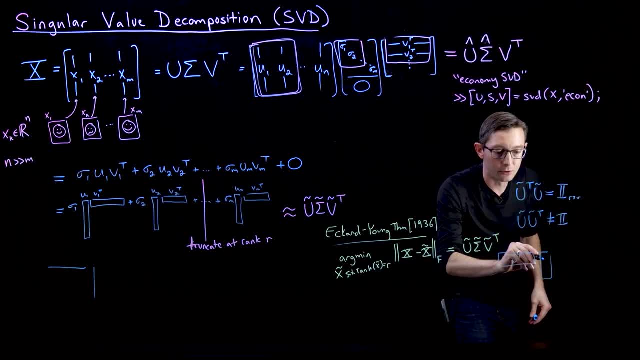 they're these kind of short fat matrix times U, tilde. These columns are still orthogonal. So if I dot product them like this, I still get an identity matrix. But now if I construct this quantity U tilde, U tilde transpose.